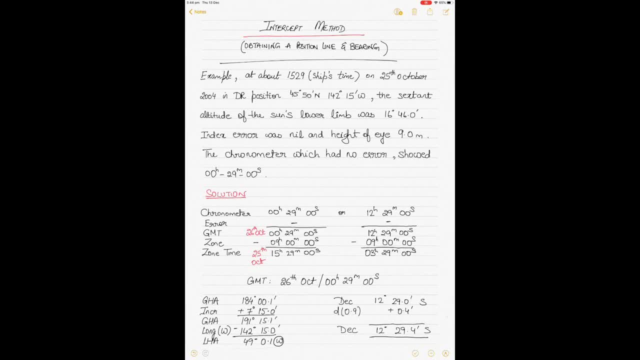 the angles at which the ship has a bearing from the celestial body. So if we can obtain a sextant altitude and if we have the other details, such as the time of the altitude and some of the other details, we can actually obtain an intercept and a position line. 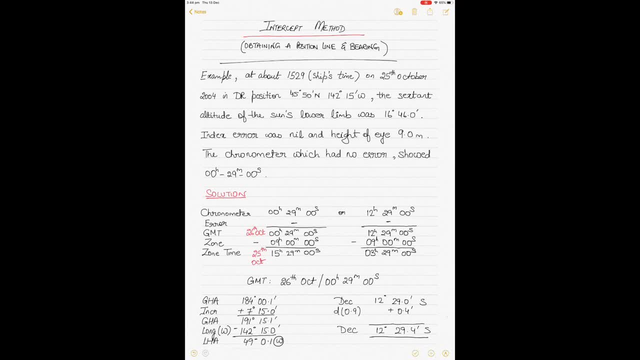 which gives us the bearing and an approximation of where the ship is at sea, and the intersection of two such position lines gives us the position of the ship. two or more position lines. so the more the number of position lines, the more the position lines. the more the position lines, the 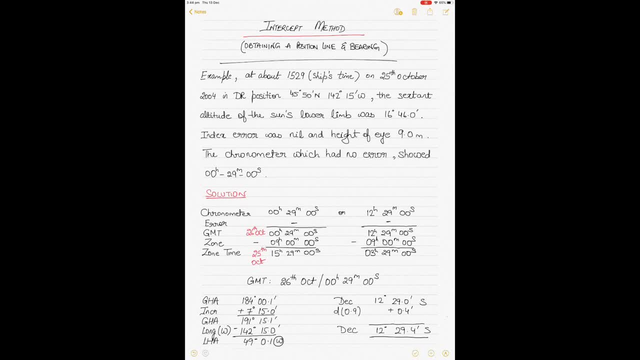 better it is because it gives us higher accuracy. Now, in this video, I will only focus on deriving the position line and the intercept of the bearing of the celestial body, and in my next video, part two of the series, I will show you how two position lines can be used to plot the ship's position at. 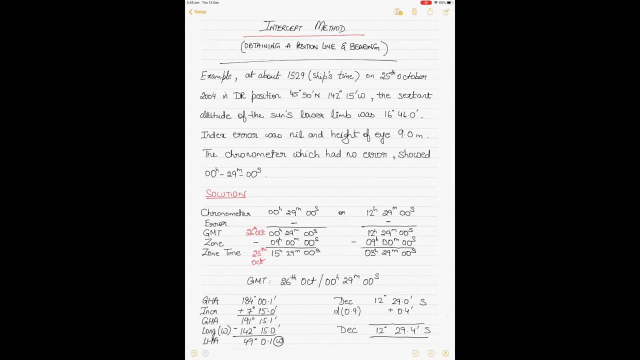 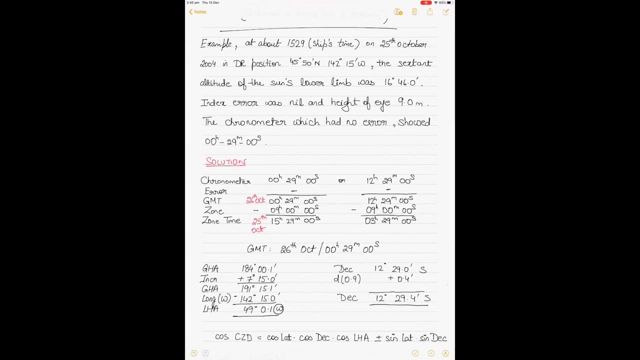 sea. All right, so we will do the plotting in my next video, otherwise this video will become a bit too long and you will lose track of what we are talking about. it becomes too lengthy and then you lose track, you lose interest. All right, so let's let's talk about the 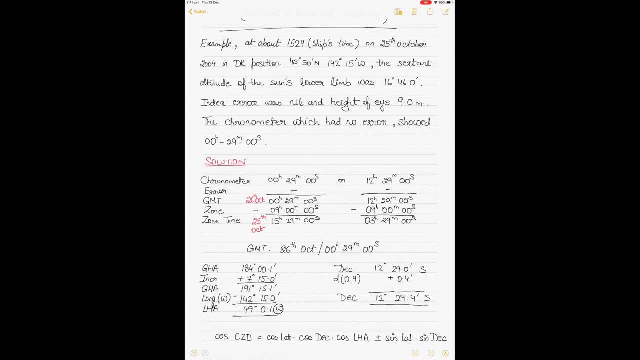 intercept method and the example. here we'll be using sun, and if you see my previous videos, you know how to derive the LHA and how to get the true altitude of the star- the planet as well. so the principle remains the same, so don't worry about it. so we use the example of the sun. it's a pretty 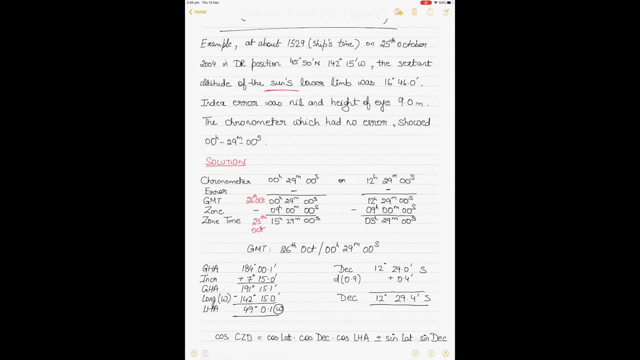 long question to solve so it takes a bit of time. so just try to hold on the interest here and if you kind of drift off, then pause the video, watch it again later on, or you watch it in sections, depends on how you want to do it. 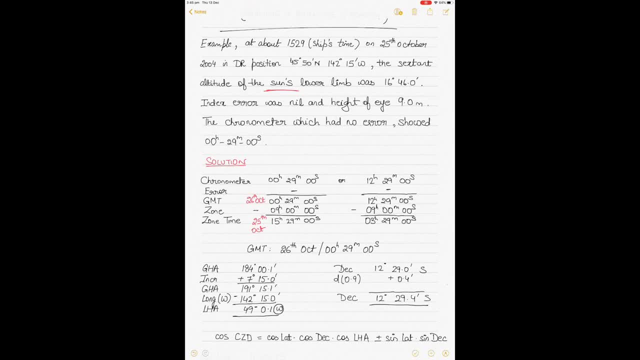 All right, so it's a bit lengthy, but let's see how you go with it. All right, so we've got the sun's lower limb as a celestial body and we've got a DR position as well, right? so the whole idea behind this is that we've got a DR position, or dead reckoning position, rather- and I've been using 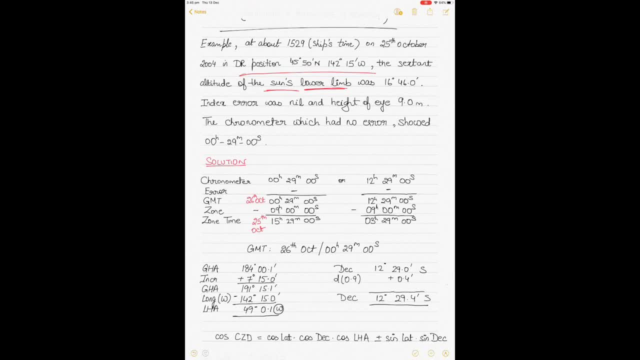 I've been saying DR position in a number of videos. probably I've never mentioned that DR stands for dead reckoning. dead reckoning is an approximate position, so we've got an approximate position. and those were the days when we didn't have GPS on the ship, so or the GPS would sometimes stop giving. 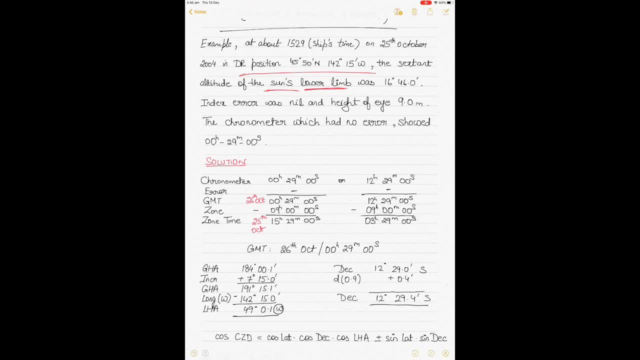 signals, not on the modern ships. the modern ships, you are getting signals. you have multiple GPS's actually, but those days you didn't have multiple GPS's or the GPS would not give signals sometimes. so you would have a DR position, approximate position, then you would use a sextant to get. 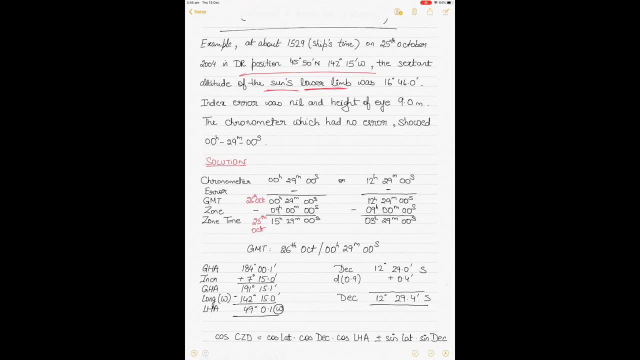 an altitude of the celestial body and from there you could plot the ship's position. all right, it used to be called the fixed position. I'll show that- how to do that- in my next video. so the sun sextant altitude of the sun was 16 degrees and 46 minutes. the index error was nil, so zero height of. 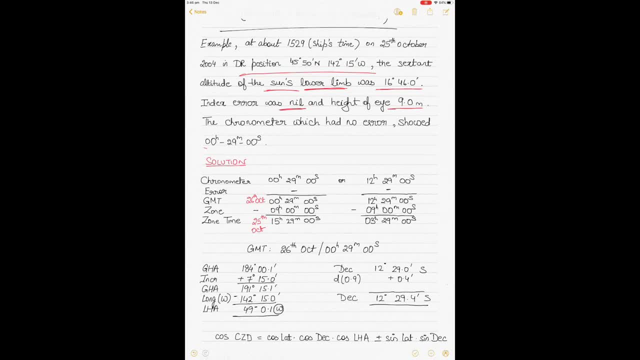 the sun was 16 meters and the chronometer, had no error, showed 00290. all right, so this is the chronometer time. to derive the GMT from the chronometer time, we need a hint in the question. the hint is given here that it is 1529 ships time on the 25th of October. all right, so this is the 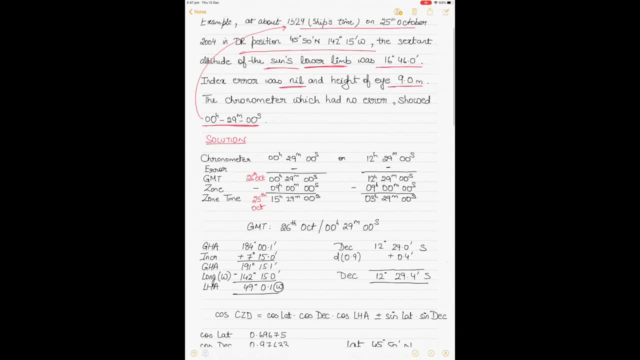 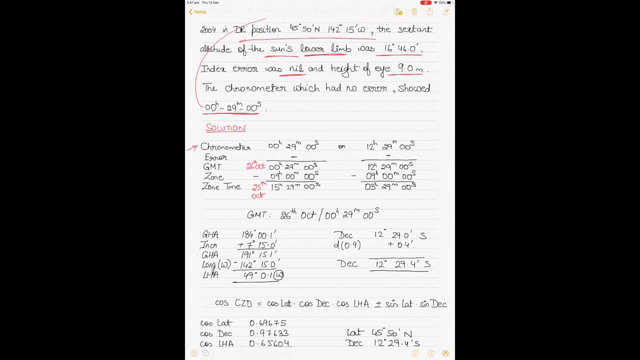 hint given to us. so let's derive the GMT time from the chronometer time. so if the chronometer is shown as zero, zero, twenty nine, zero, zero, zero, so the chronometer pretty much looks like it's going to look like an analog watch. now, of course, on the ship we can get an idea of what the time is, whether 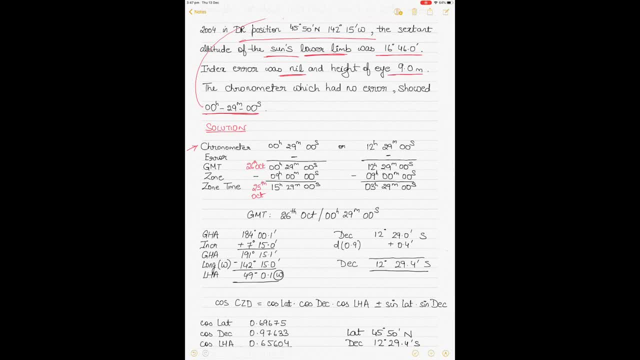 it's zero, zero or twelve hours, but for academic purposes here, or for numerical purposes, we are not really sure that the chronometer time zero zero could mean zero, zero in the early in the morning or twelve hundred hours in the afternoon, so we need to derive the GMT from there. so because 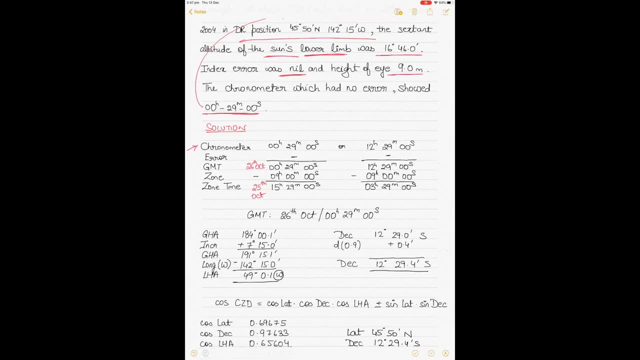 the error is nil of the chronometer. the GMT time is same as a chronometer time at 0029. now we need to derive theяв, the code and the MUD, which means we need to have some kind of data, chan, api- and we need to derive that. we need to have what you know, you want, the mismatch condition. 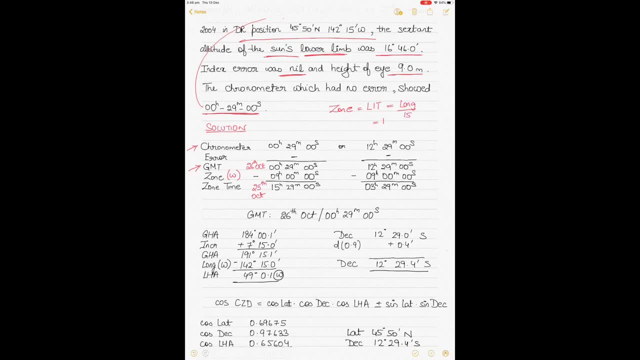 we want the present general, so unrest time. so basically, what we need to do? what we need to do is our instruction. so the time loved, so 15 than june. so in which order we will write: 2 oh x is the length of the Twilstar, so I will simply write 15 and then I will write it out. you do not feel, 취 GPS? 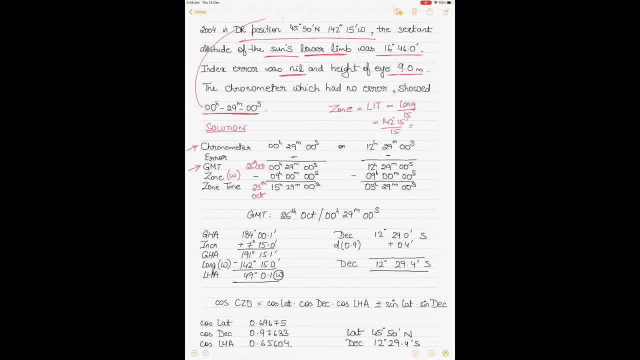 142 degrees, 15 minutes by 15, what you will get is, as 142 degrees and 15 minutes divided by 15 is 9 hours 29 minutes, so 9 hours and 29 minutes. now, since this is less than 30 minutes, the zone would. 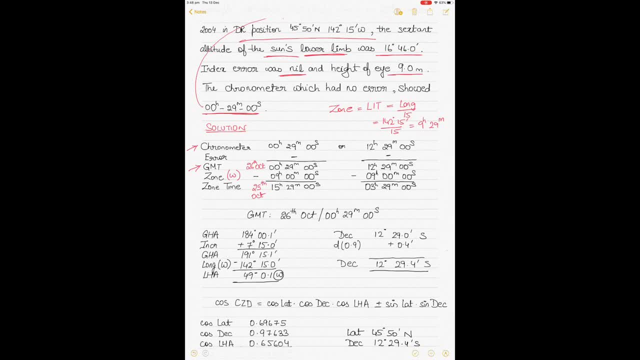 be 9 and because we are in the west zone, the west zone that means gmt should be ahead of us, so the time on the ship will be behind gmt. that's why we subtract it now in both the cases when we subtract 9 hours. in one case we get the zone time as 15- 29 and in the other we get the zone time as 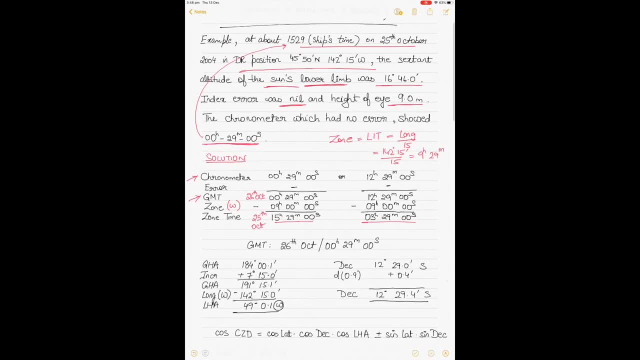 0329. now this is where the hint comes in handy. now the question says: or given the hint given in the question is that it's 1529 ships time on 25th of october. so immediately i know that this second case is not the correct case. i will cut it off because the zone time here is 1529 as well, and 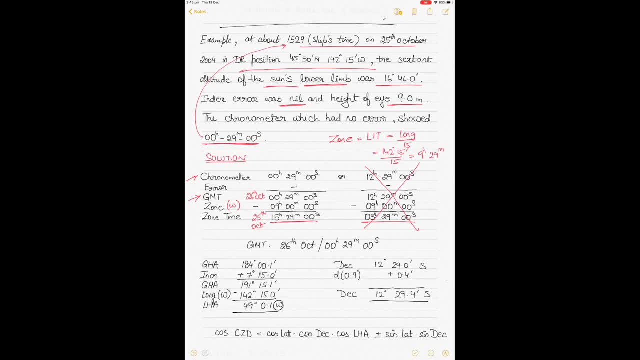 it's 25th of october, but because we are behind gmt and gmt is nine hours ahead of us, that means gmt on the. at gmt the date has already changed to 26th of october and that is why your gmt is on. 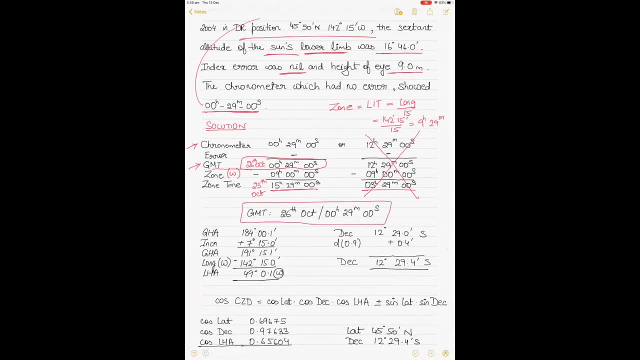 the 26th of october 0029. right, because your ship is in the west longitude. gmt is on the greenwich meridian. they are ahead of you in terms of time. they are nine hours ahead of you. so basically, it's 25th october, afternoon 1500 on your ship, but it's already midnight past midnight on the 26th. 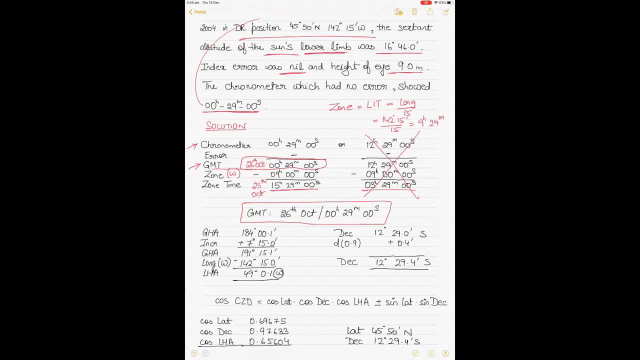 of october at the greenwich meridian, whereas i have explained this before. watch this part again if you found this a bit confusing. but remember to use the hint given in the question to get an indication of what the gmt would be, and remember the rest of the question has to be done using the gmt time and not the zone time. 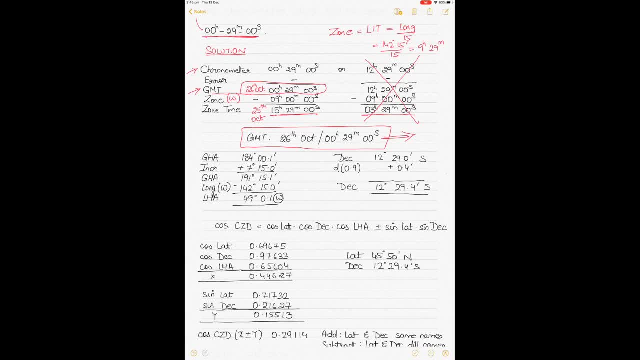 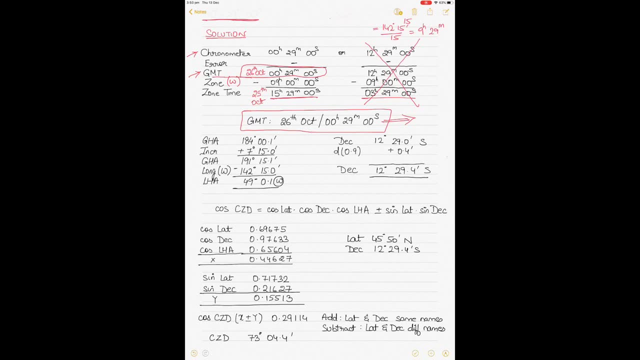 many, many, many people make the mistake and they use the zone time for further calculations. don't do that. use the zone, use the gmt time, all right. that's why i i've written it in a box and highlighted it, to make sure that you don't use the incorrect time, all right. having said that, 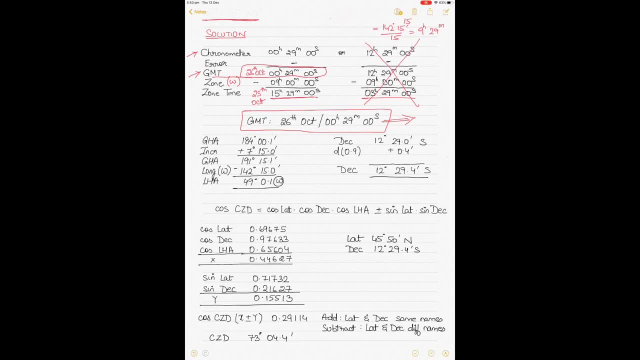 now we have to not go to the almanac. i have shown in my other videos how to obtain the lh and declination of the sun, so i won't waste too much time about on it. so what i will do is i'll quickly show you that the gha for the 26th of october for the sun at 00 hours. so you can see this is 26th of. 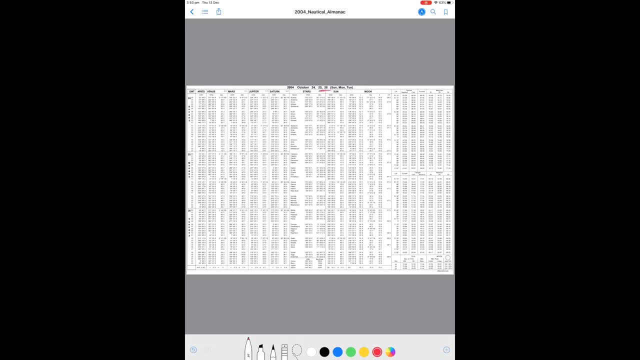 october. uh, right here. uh, the sun is right here. 00 hours is right 20. we need the 26th of october, right? so 26th of october at the bottom here. so here your gha is. this is where your declination is. uh, this is your d value, right? so these are the values. 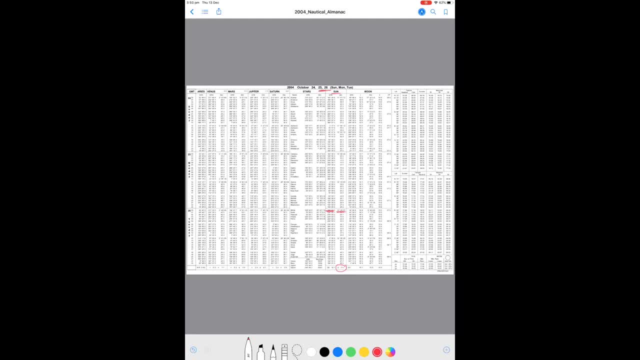 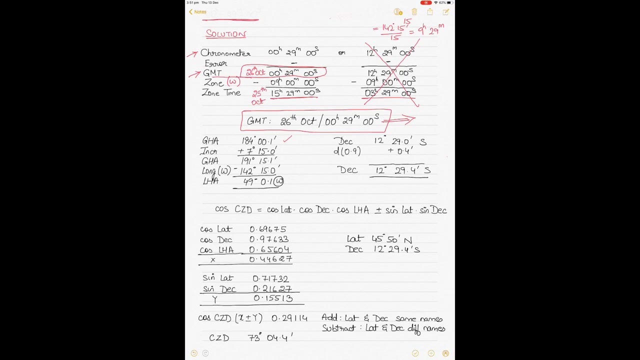 that you will be using to get your gha and declination and d value. uh, or else watch my other videos where i've explained in detail what to do with these values. so i'll quickly go back now and i'll continue with my calculation. so these are the values i've used, the increment value. 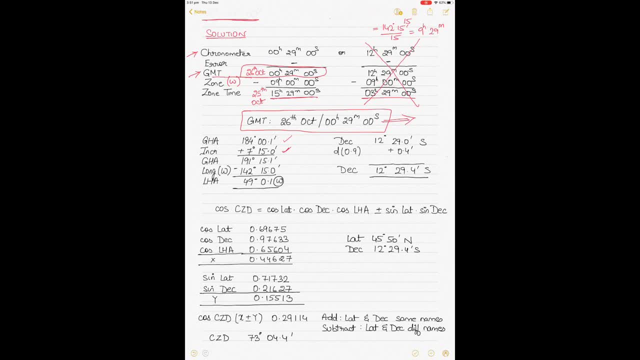 is obtained from the increments page in the nautical almanac, and i'll quickly show you what it looks like. so we need the increment for 29 minutes and zero zero seconds. right, this is for zero zero hours, and so the increment for 29 minutes, zero zero seconds. uh, let me go back. 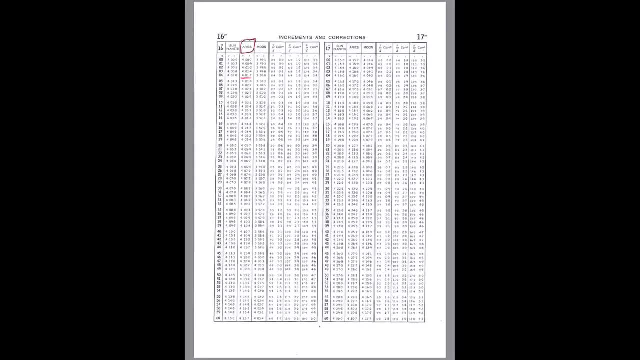 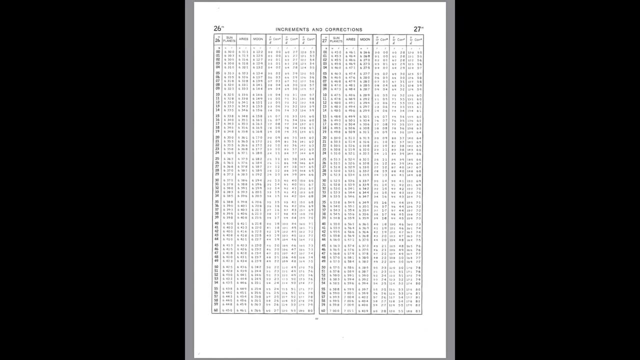 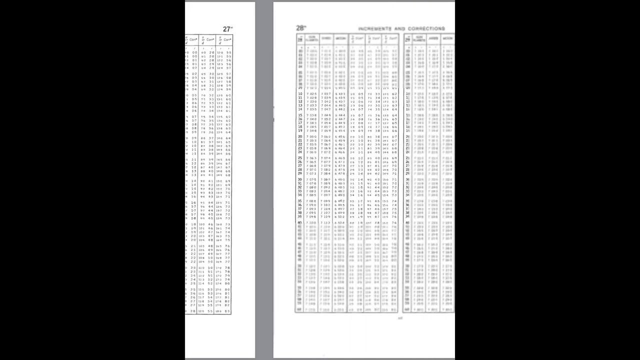 here and if i go back here so you can see that for 29 minutes. so 26, 27 0 0, 26 is uh here. is that right? for what? the time was uh, it was uh 0 0 29. i'm sorry, not 26, but 29 right. 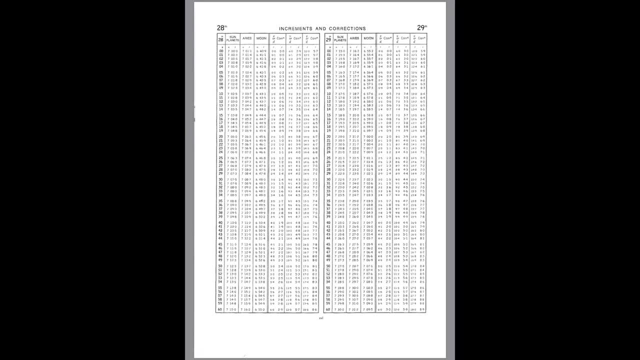 so for 29 uh increments, for sun is here. okay, bear with me, this is a painful process that i take you guys through, right. so this is the 29 minutes column. this is the sun. this is the zero second. this is where the increment is uh you get. 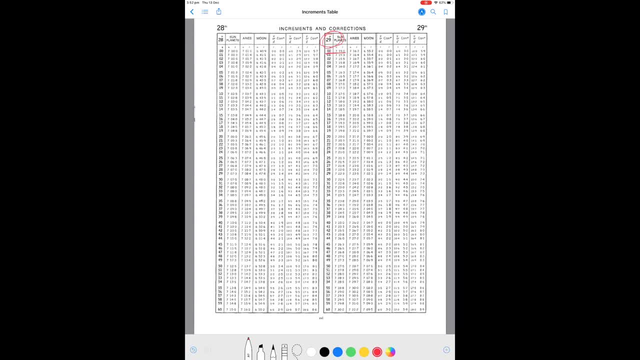 the d value for 0.9 and uh here 0.4. the declination was increasing, so will add it. so i've explained all that to you in my previous video. otherwise, just watch my previous video where i've shown you correction of altitudes and then you can get an idea. so i don't want to waste too much time here on getting these. 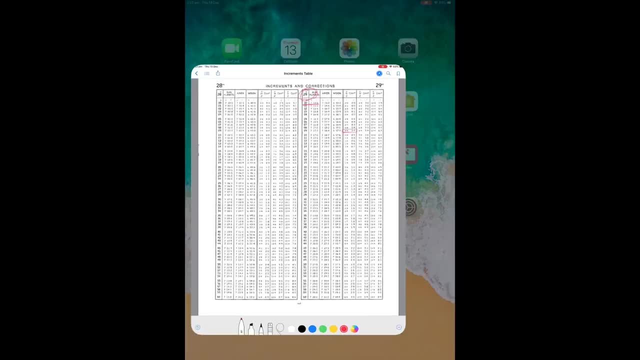 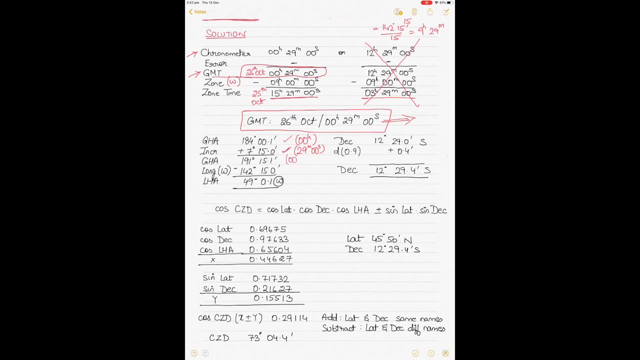 but i just quickly showed it to you on how to get the increment and the de-correction value for the declination. so i go back here and you can see that i've put in the increment here. this GEC is for zero zero hours 29 minutes and zero zero seconds after focused on human adult soldiers. so again, if 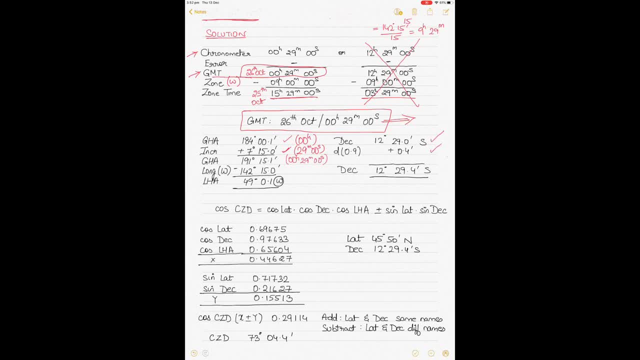 it showed よ то this妈 argument. shown you, if you might�몣. after applying the correction, you can see the declination is applied as well. so I've got the declination here. the longitude in this case is west longitude. west gha would be best, I would. 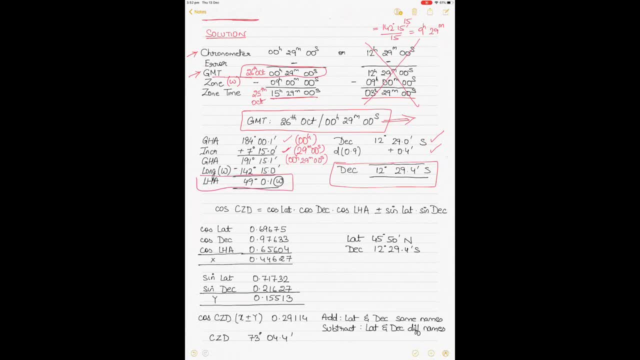 subtract my longitude to obtain my lha right lha value is less than 180, so I have named my lha 0 to 180. so the rule of thumb is 0 to 180, you name the longitude west and if it is greater than 180, 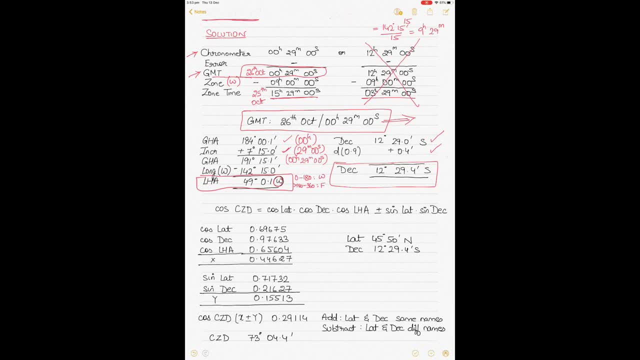 to 360. you name the, not the longitude, sorry, the lha. you name it east. all right, in this case it's less than 180, so the lhas will be named west right. so if your longitude is west, gha is less. so we subtracted longitude from the gha to get the lha value. we've got the declination. 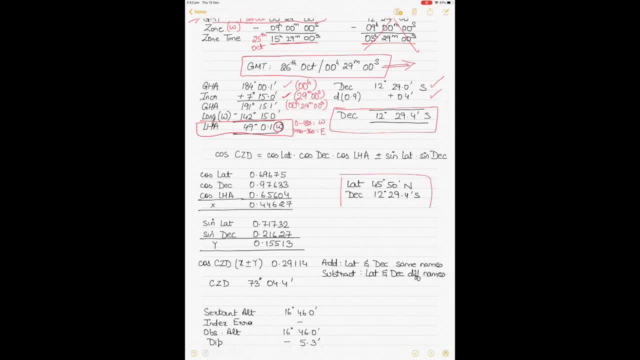 and we've got the latitude as well over here, so I've recapped it over here, right? what I want to focus here on more is this formula: here, this is the formula that we use to calculate something called czd. now, czd stands for calculated zenith distance. calculated zenith distance. 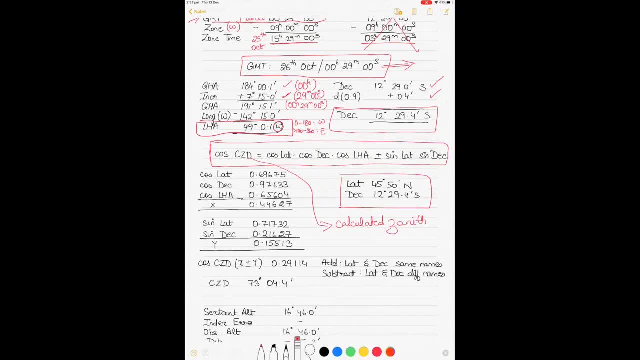 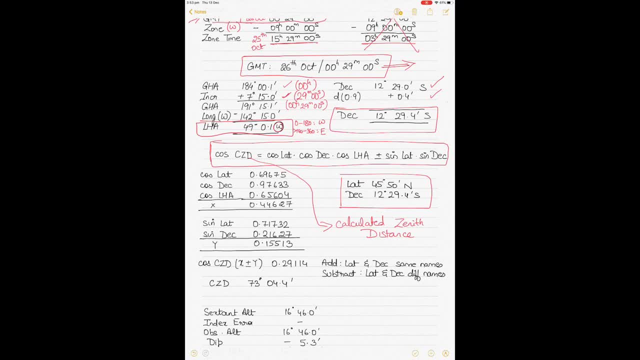 dec times, cos of lha, depending on the names of the latitude and declination. you then add or subtract it to a product of sine of lat and sine of declination. so you can see, here I have worked it out here, you can follow me here. so cos lat value is 0 to 180. so this is my terrible handwriting. 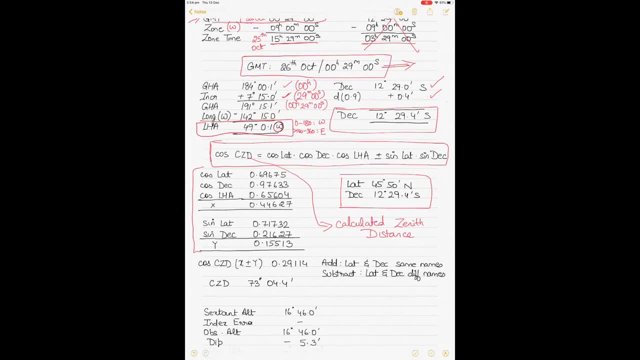 and then the value of the latitude and declination is additional values here. so a product of these three gives me a value called x. now I have stuck to five decimal places because it pretty much gives you a good accuracy. don't use two decimal places. try to use three to five decimal places. that gives 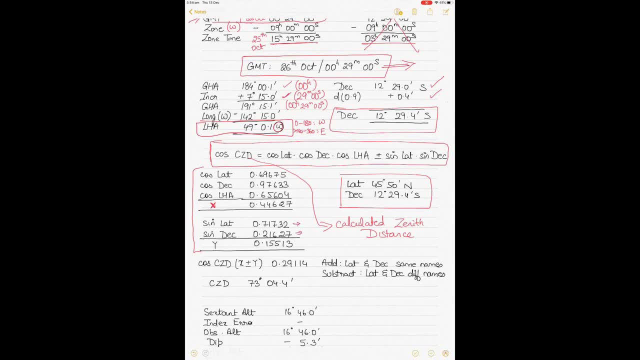 you better accuracy, all right. and then I've got my sine lat and sign declination value as well. a product of these two gives me my y value. now, whether I need to add the x and y or subtract, it depends on the rule. that are same names, I will add them. right. the rules are given here, if there are. 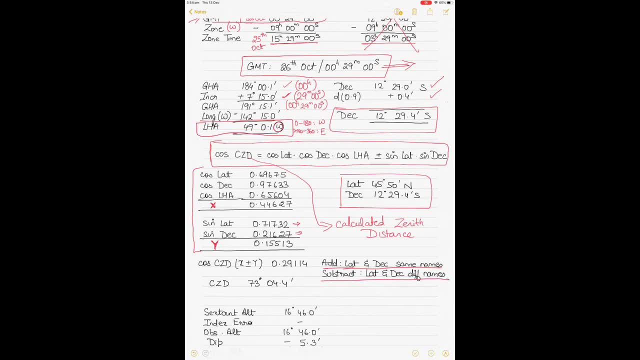 different names. I will subtract them now, in this case, here, because the latitude and declination are different names, one is north and the other one is south. I will subtract them. that's right. so that's what I've done. I have subtracted X from Y, so what I will do is I will delete the plus sign then, so it makes it. 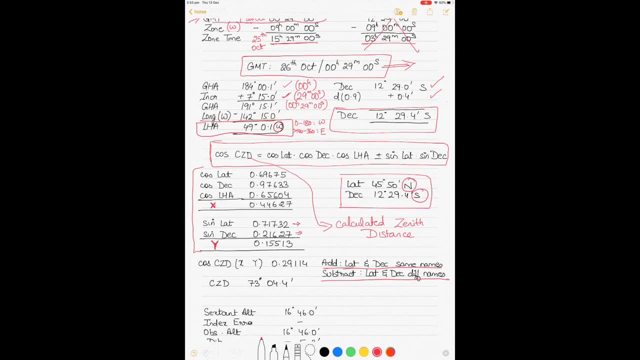 easy for you, right? so what I will do is I will subtract it and a cos inverse of this value, a cos inverse of point zero. point two: nine: one one four will then give me a CZD, or a calculated Zener distance of 73 degrees. four. point four: 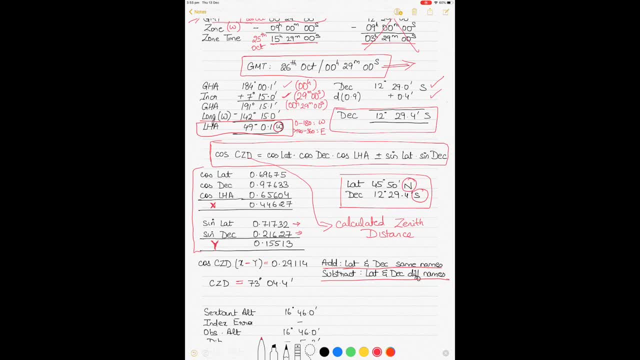 minutes. all right, so see the for the formula above. that shows the formula for cos, CZD, and you know how to do that, right? so just try to match your values with mine. make sure that if they are not matching, you reach at your values, because mine are correct, I can tell you that. all right, so once we've got a CZD, 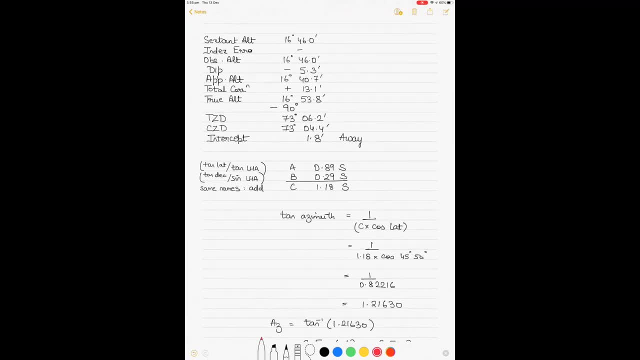 or calculated Zener distance. we need to calculate a two point zero point two. nine one four will then give me a CZD or a calculated Zener distance- any distance, and we calculate a two Zener distance from the sextant altitude. I have shown my separate videos how to do that as well. it's pretty. 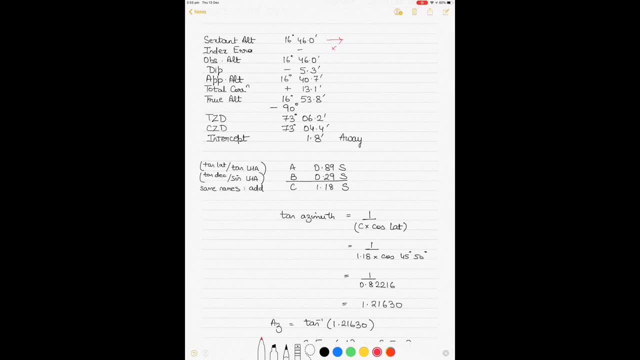 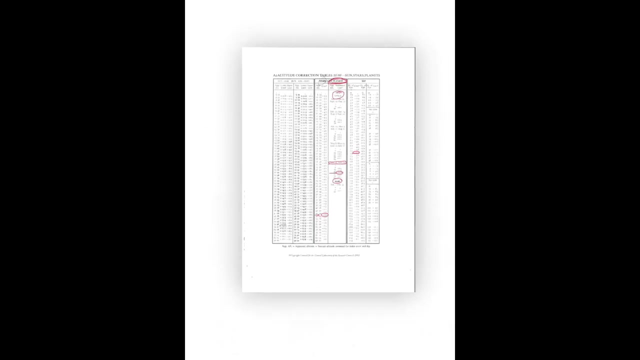 straightforward. you've got your sextant altitude index. error was nil. from there. you get your observed altitude. then you apply your height of I correction from the height of I tables. your height of I is, in this case is nine meters. so if I go back into my nautical almanac and I go back on the first page of the 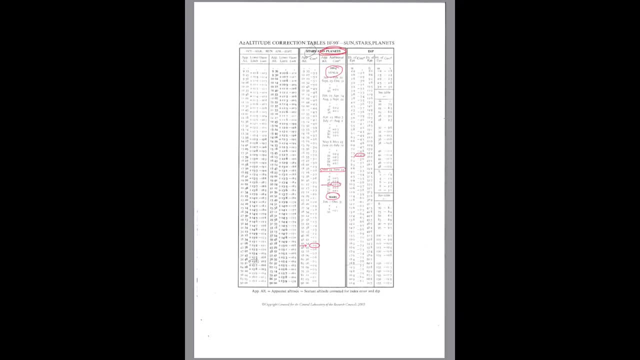 nautical almanac you can see here is that my height of I is given you in a minute. that's right, I've got it here. so my height of I is given here. it's the dip is the height of I and let me erase the rest so that you guys don't. 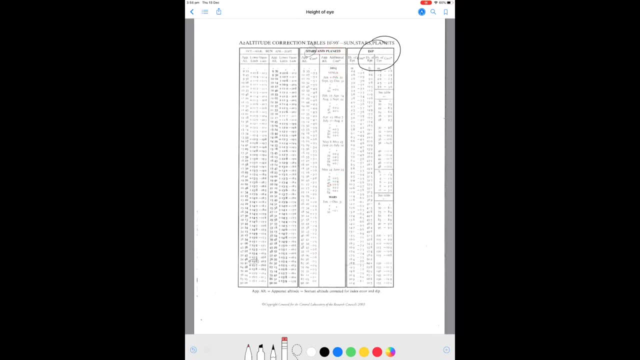 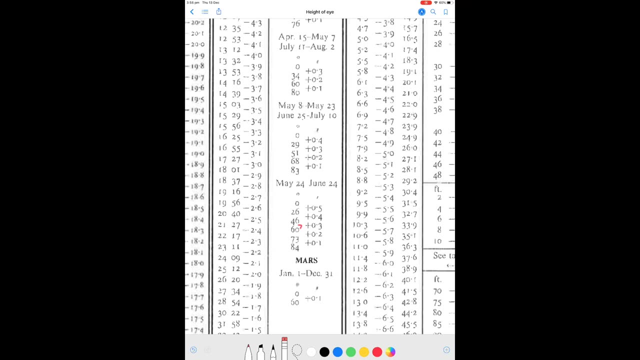 get confused with what we are doing here. so height of I or the dip table is given here for nine meters. if you go down nine meters and if I, if I kind of zoom in, you can see for nine meters, the correction would be somewhere here which is minus. 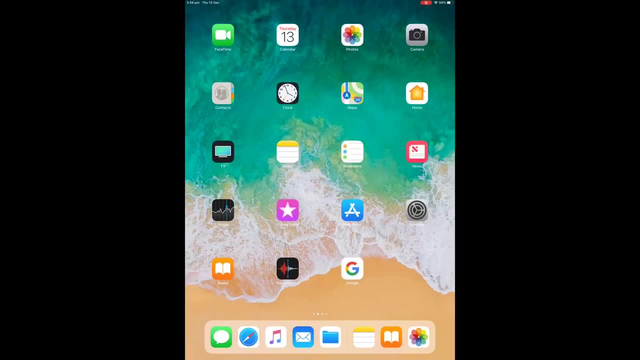 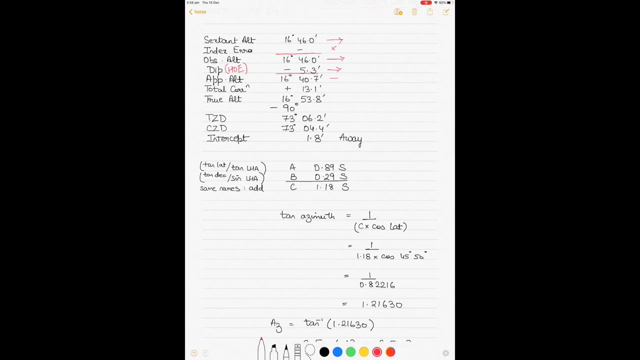 5.3. all right, so I'm not going to waste time, too much time here. I'll quickly go to the calculations so you can see that that's the height of i have used is minus 5.3. a subtraction gives you the apparent altitude. taking the apparent altitude, we go back to where we were. 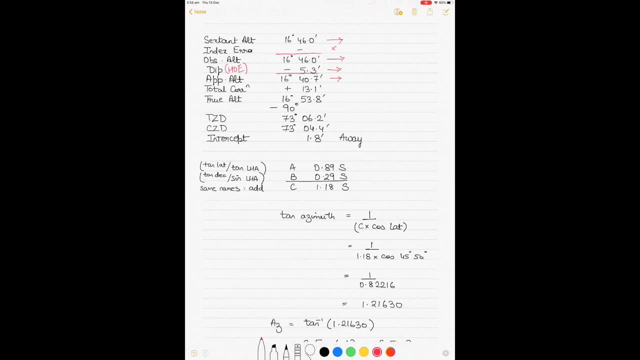 we found our height of i4 for total correction. total correction, so apparent altitude is 40.16 degrees 40.7, and it was a sun's lower limb. it was the month of october, all right. so i've explained all these things before in my previous videos. at the risk of repetition, i keep repeating myself. 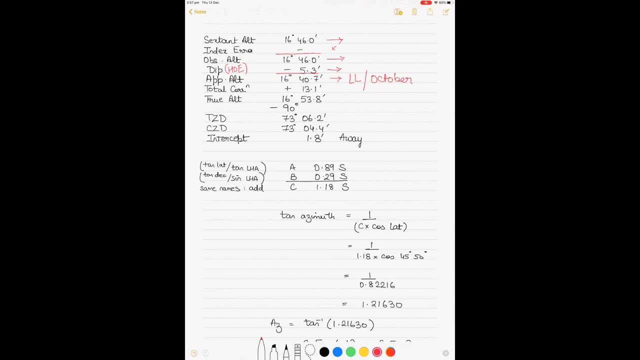 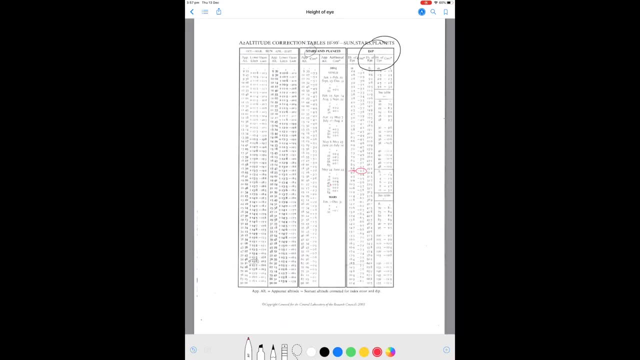 watch my other videos where i've shown you how to correct the sextant altitudes to obtain the true altitude. all right, so i'll show you what to do with this. go back to the page from where you get your height of i from. uh, this site here gives you the total correction for the sun, the month is. 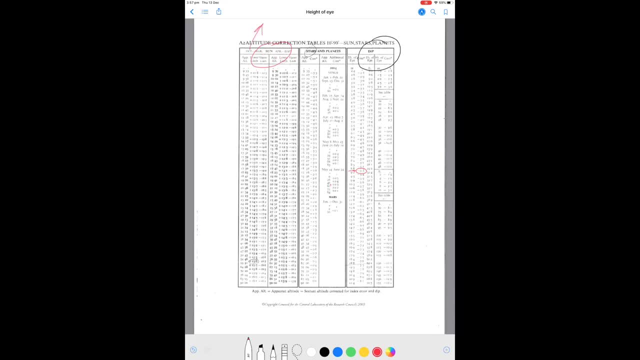 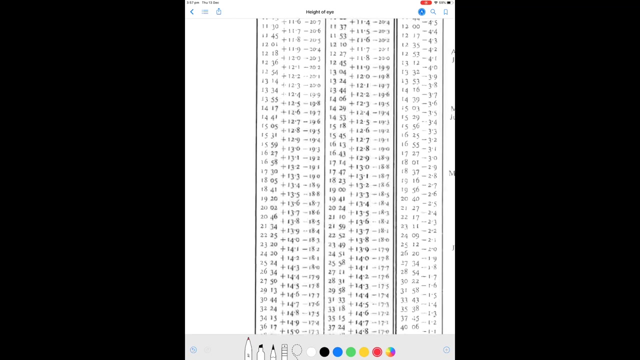 october, so it should be somewhere here. the altitude or the apparent order to the 16: 16 degrees 40.7, it's the lower limb right. so we have to go down the lower limb column, which is this column here, and if i zoom in here, 16 degrees 40.7 would be somewhere here. the correction should be plus 13.1. 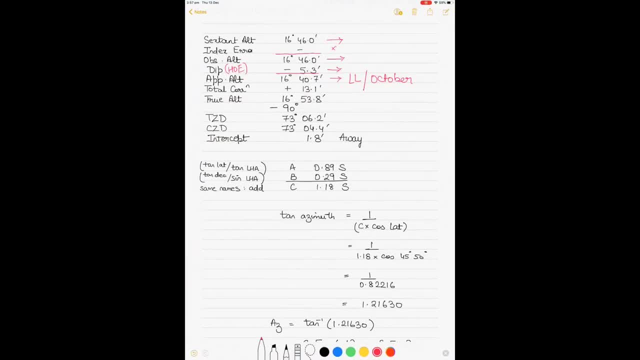 so that's how i got my correction from. so and that's what it says here: 13.1: right, i will add the correction because it's lower limb. once i get that, once i get my true altitude, i subtract it from 90 degrees to get my chosen distance, because true zenit distance, or pzd, is equal to 90 degrees. 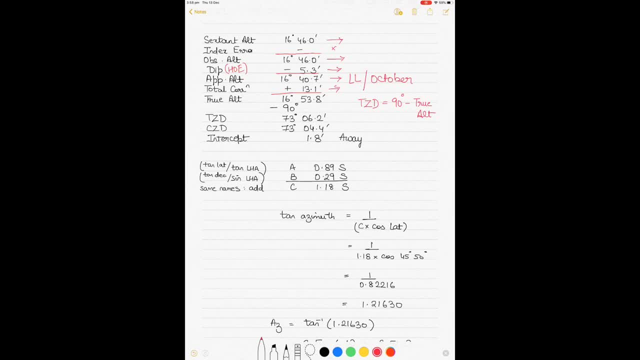 minus true altitude. all right, once i do that, i get my true zenit distance, which is tzd. true zenith distance. that's what it stands for. all right, in case my pronunciation wasn't very clear. now what i have to do is to calculate my intercept. i have to compare the true zenit. 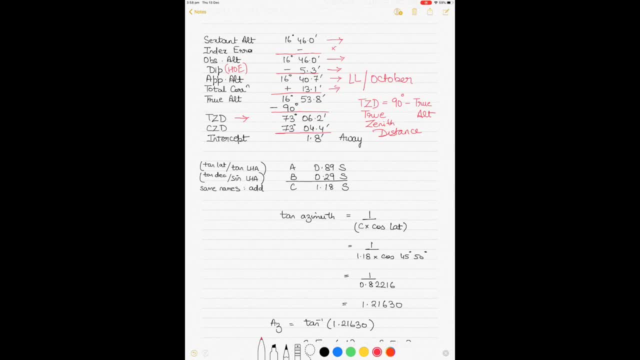 distance to the calculated zenit distance. all right, and there's a rule of thumb again. now there are a lot of rule of thumbs. i teach you guys. so, yes, there's another rule of thumb. i'll i'll erase this and i'll write it next to the values here. so the rule of thumb is that if you 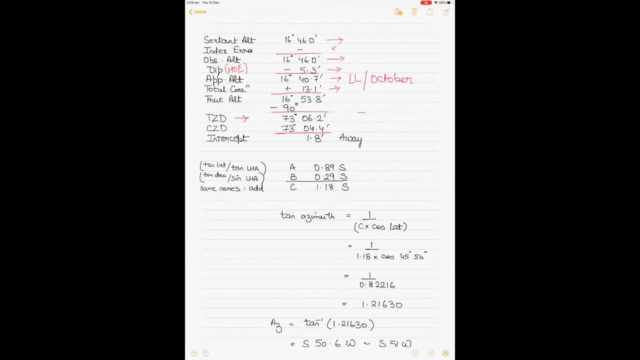 compare the truth and a distance with the calculator, zenit distance. and if true is less or true is tiny, then the intercept is named two words. so normally we call this rule t t, t, true, tiny, two words. so if true is less, or true is less than what? less than czd right? 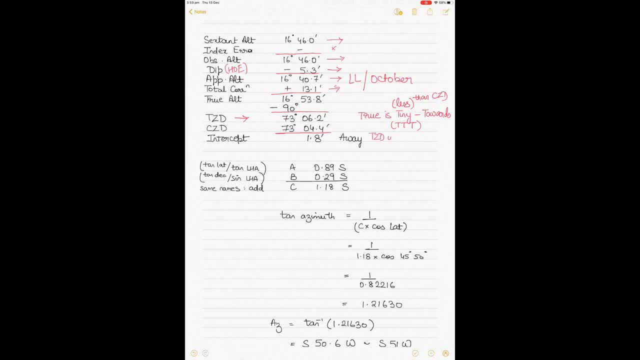 and of course, if true zenit distance is more than czd, then you name it away. so you have to remember the top one, the trip, the triple t, two, two, tiny two words. that means if true is less than czd, it's called two words. but in this case you can see the true zenit distance is. 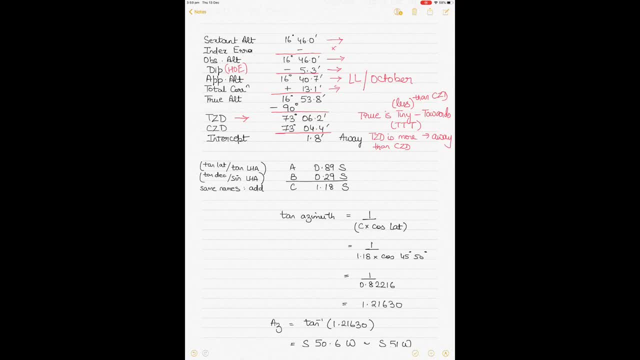 more than the calculated zenit distance, and that's why- and the intercept is the, of course, always the difference between the two, and the difference between the two is 1.8 minutes, and the naming is away, so it's 1.8 minutes away. right, with that, you got your intercept, so one problem solved. 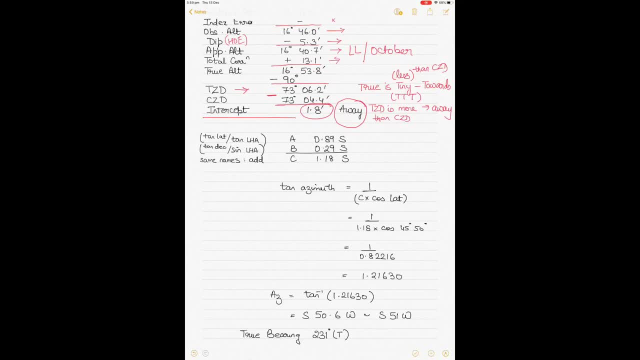 all right, later on i'll show you how to plot this. i mean, towards the end of the video i'll show you how to plot this. but how to use this to plot the shift's position will be shown in the next video, where i'll show you how intercept is used to plot the ship's position on the chart. all right, so note. 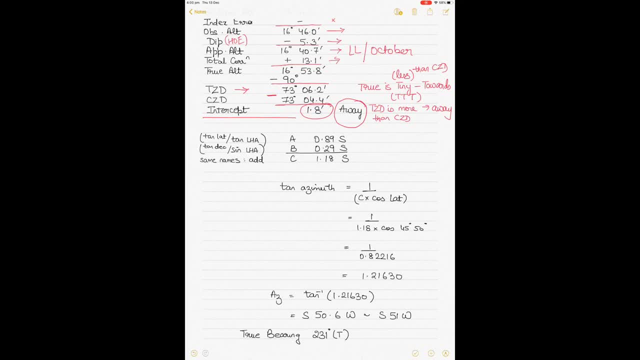 on this intercept, don't forget this intercept. and then what we do is what we have done before. in this example, we have calculated our compass errors. we calculate the components of the bearing a, b and c is calculated as tan lat divided by tan of lha. straightforward stick to two decimal places. this: 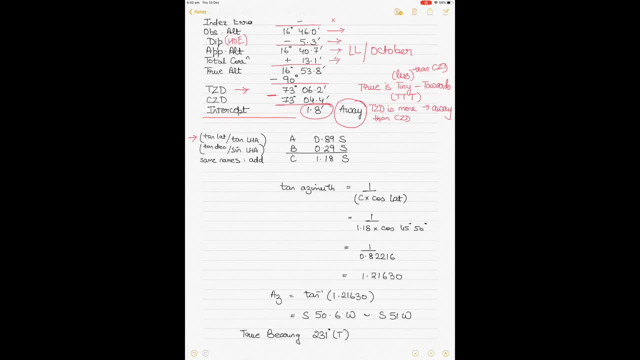 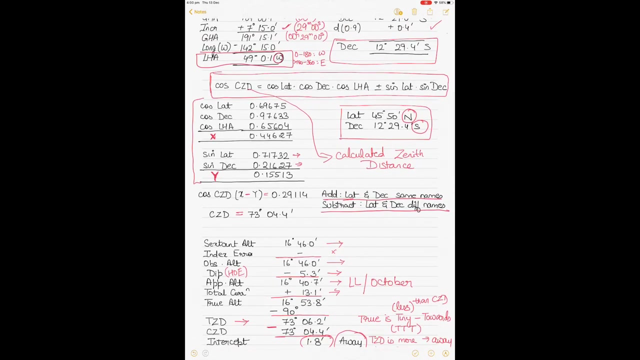 time. you can go to more, of course, but i see two decimal places when it comes to a, b and c's you name it opposite to latitude, unless it's always named opposite to latitude, unless lha is between 90 and 270.. in this case, is lha between 90 and 270. let's check what's the lha. no, the lh is 49. 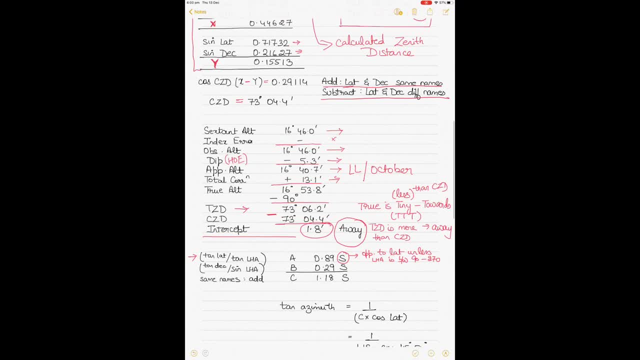 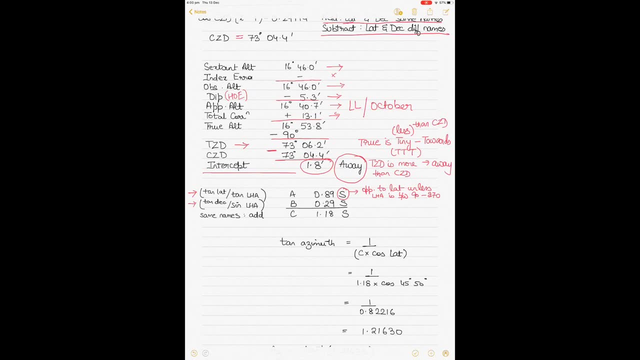 degrees, so it's not between 90 and 270. so it will be named opposite to the latitude, and latitude was not, so we'll name it south right. then we calculate the b component. b component is calculated as tan declination divided by sine lha. i've written the formulas here so that if you don't understand what. 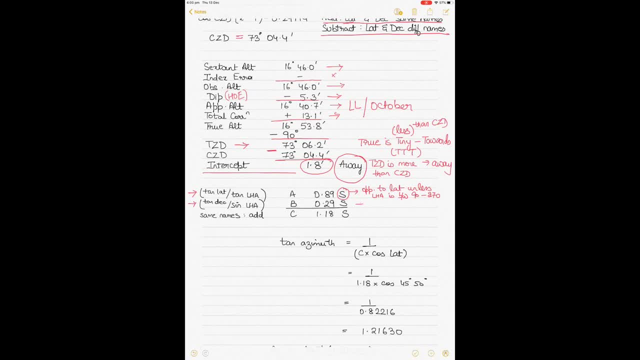 i'm saying, at least you can follow what i've written and you name it same as declination. now, in this case, of course, the declination was south, as you remember from before, and that's why i named it south. right now, how do you get your? 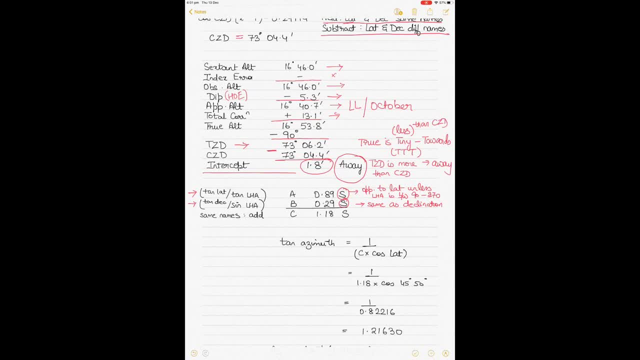 c component. your c component is depends on a and b, so if they are the same name, such as south and south or north and north, then you will add them. otherwise you subtract them. in this case, of course, they are the same names. so you add the two and you get your c component and you retain the name of. 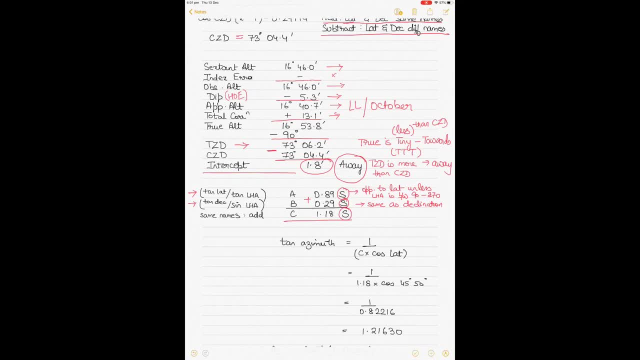 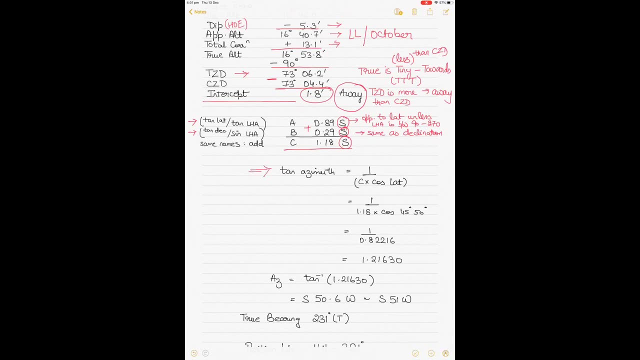 the, of course, the larger, but in this case, both of them are south, so it will be south, all right. why all this is important? um, you will slowly sleep. once you get your c, you calculate your azimuth. how do you do that? you use this formula here: tan azimuth equals one by c times. 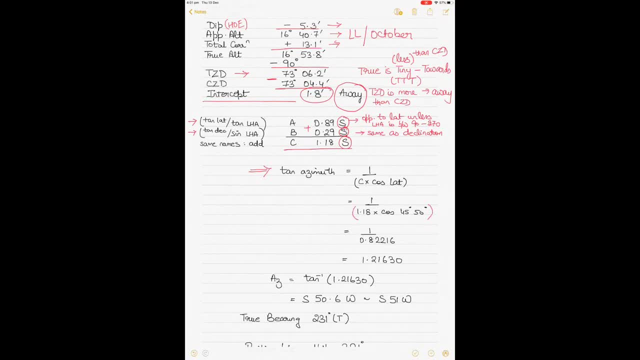 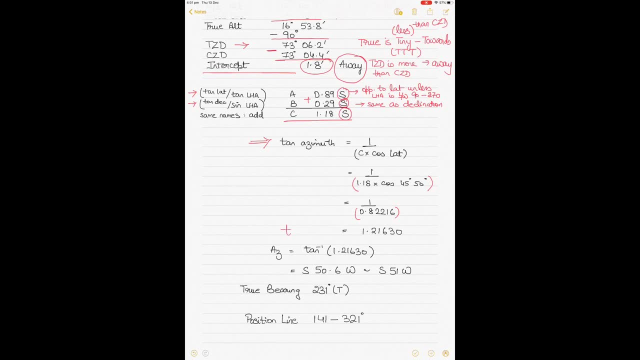 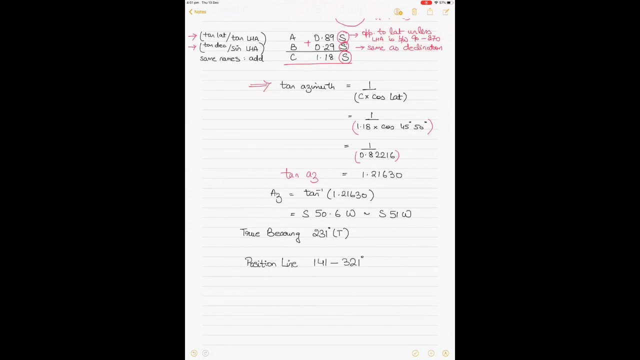 coslet. find out the value of c by coslet first, before you divide one by it. all right, just the way i have done it once you get this. so your tan azimuth here equals 1.21630. so a tan inverse of this now will give you the. 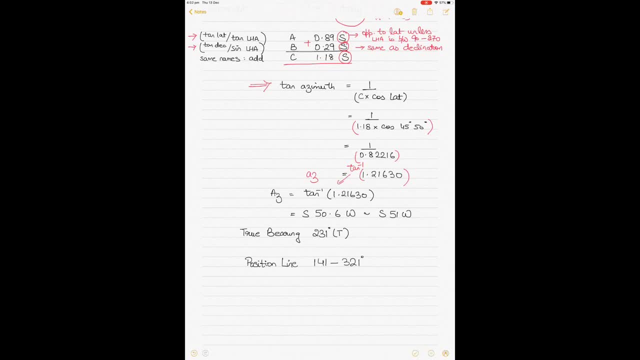 azimuth value. right in this case, again after: this is what i've shown here, so i don't need to repeat myself. so i just delete this here, right? so a tan inverse of the value gives you your bearings. now your bearing in this case is 50.6. is what you get in your calculators. now you better round it off. 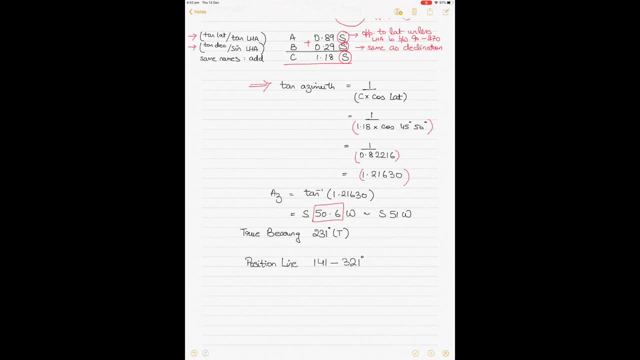 because it's a bearing. so it will be difficult for you to not not only difficult, but kind of an approximation or, in practical, to plot the bearing on a chart in decimals. you can't do that right, so just round it off to the next number if it's more than 0.5. so in this case i have named, rounded it. 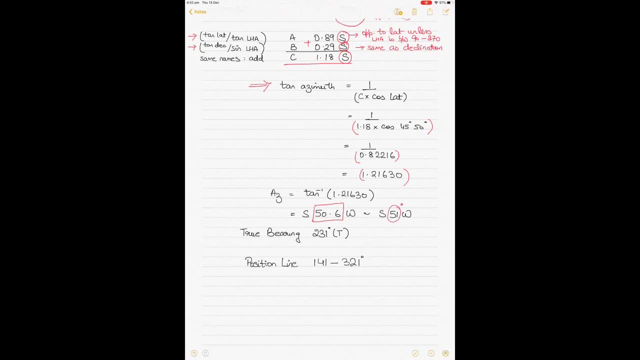 off to 51 degrees. now where do i get my south and west from? well, i get my south from the name of c- remember c, i named it same as c- and west. where do i get it from? from my lha. so if lha was between 0. 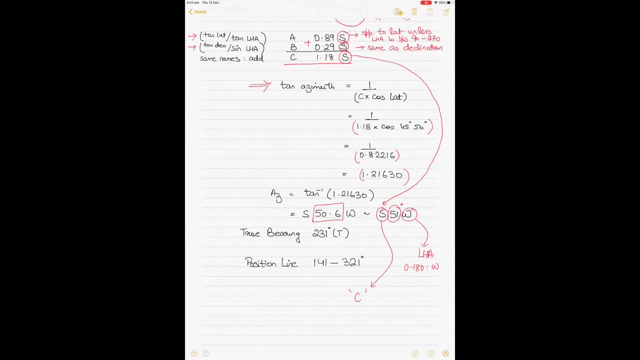 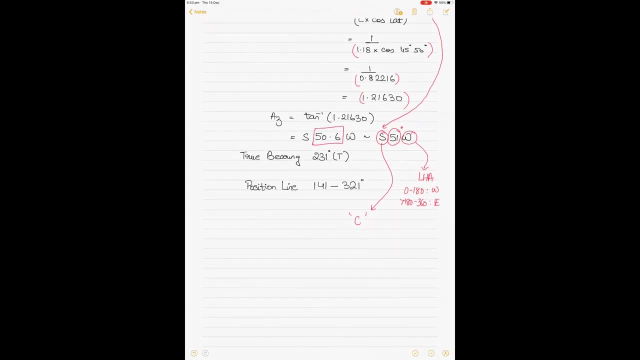 to 180, i named it west. in this case it was west because it was 49 degrees, and if it would have been more than 180 to 360, i would have named it east. so if it's south, 51 west is my azimuth- my true bearing becomes 231 degrees. true, how is that, you ask me? well, this is how it's done. i have 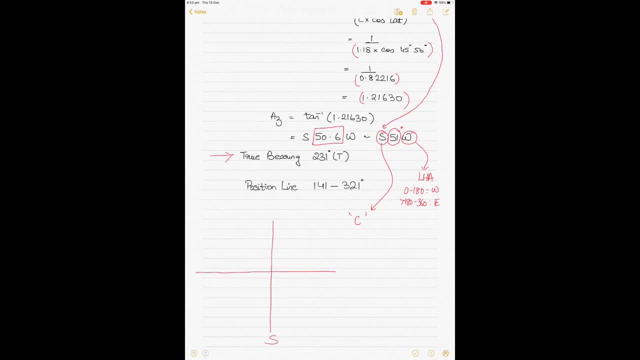 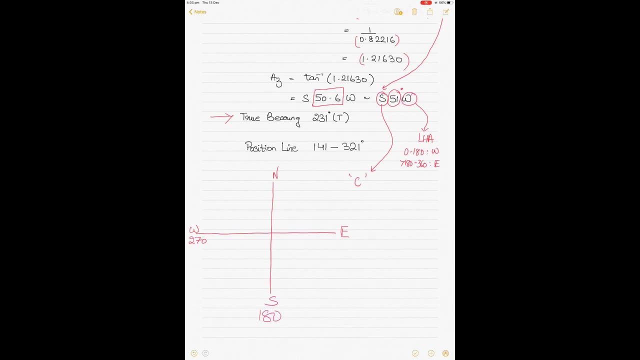 shown this in my other videos, but i just repeat this again: this is south and this is west. right, this is north and this is east. this is 270 and this is 180. so if i'm south, 51 west, that means i'm going something like this: i will add 51 to 180 to get my bearing. so 180 plus 51 gives me. 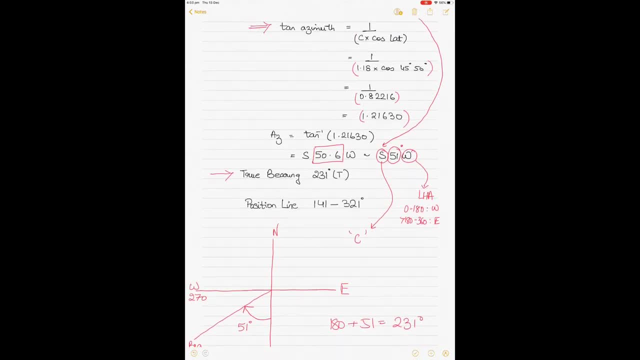 231 degrees. true, that's what i have as my bearing here. once i get my bearing as 231, i need to get my position line. a position line is a line perpendicular to your bearing line, so a line perpendicular to 231 degrees, true in this case. so how do you get your position line? just add 90 to. 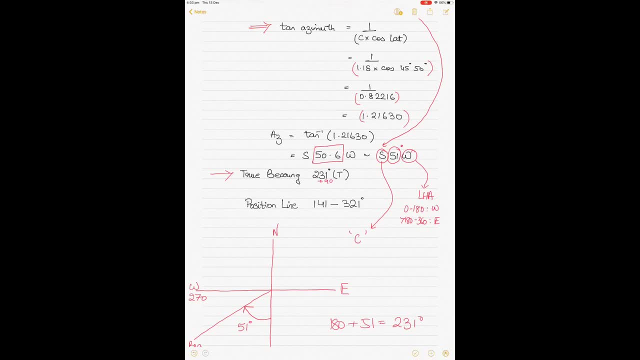 it when you add 90 to it. what do you get? in this case, you get 32. and if you subtract 90 from it, what do you get? you get 141. that's what you do: just subtract and add 90 from the bearing and you will get your position line. now, what does this mean? is this: 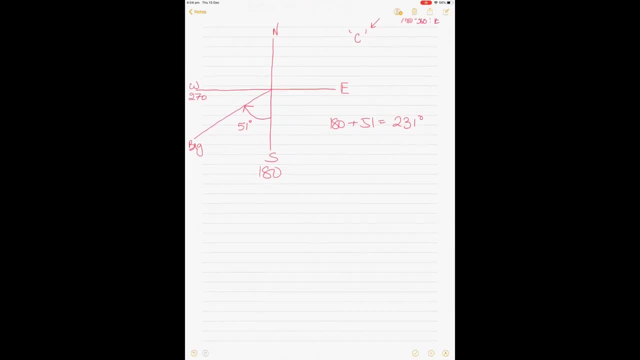 this is what it means. so, basically, you are in a dr position. let me show you what this means. this is your dr position, right, let's see now. ideally, this is what it means is that you obtained a bearing of 231 degrees. true, right, yeah, and an intercept of. remember the intercept we calculated. you should forget the intercept we. 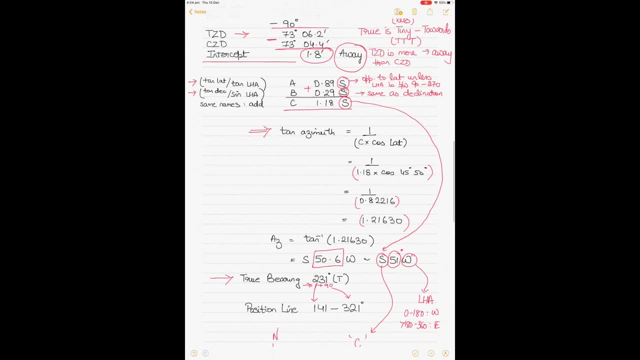 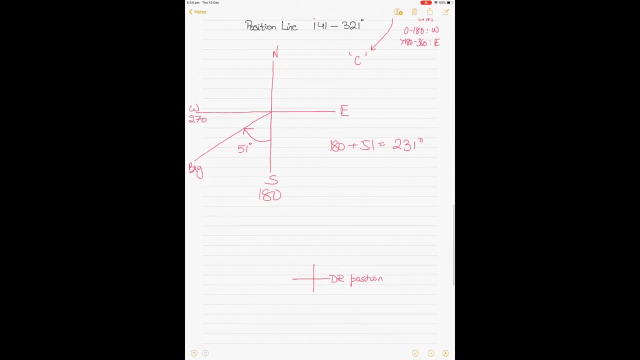 calculated here it is, the intercept is 1.8 minutes away. so when we say away, that means we are away from the bearing. so if the bearing is 231, we should go away from it. that means if the bearing is 231, we go away from it completely, diametrically opposite to 231. degrees is 18 minus 180 is 051 regys. so interception value of 0,05. 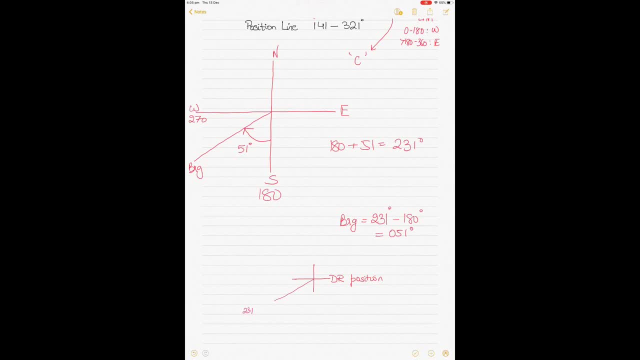 instead of going towards 231, i will not go towards 231, i will go away from it by 180 degrees. i will go 051. i am going in the direction of 051 degrees, true, and i measure 1.8 centimeters. 1.8 miles, rather, is the intercept. so this is, say, example, one point: this is 1.8 away. 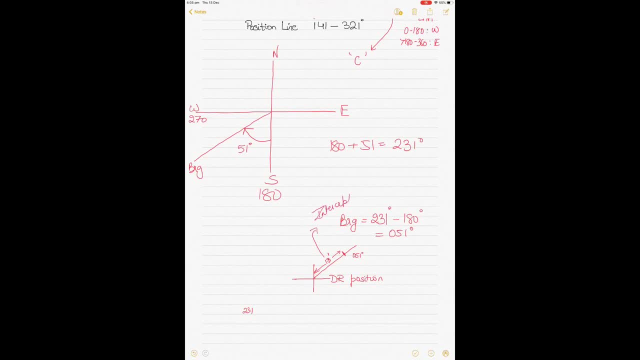 this is the intercept right: 1.8. now, when i cut 1.8 here and i draw a perpendicular line here, denoted by single arrows, it shows my position line. now this position line is 1412321. all right now. the good thing about this is you can watch it again if it was a class i. 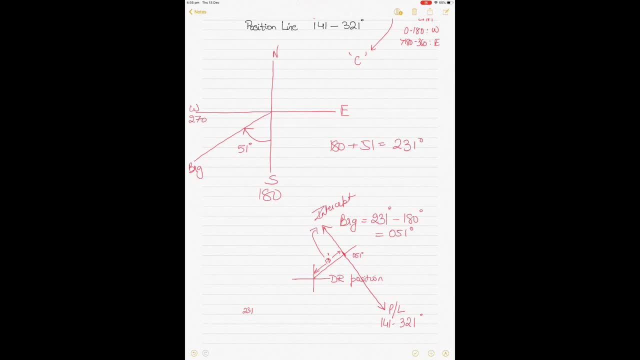 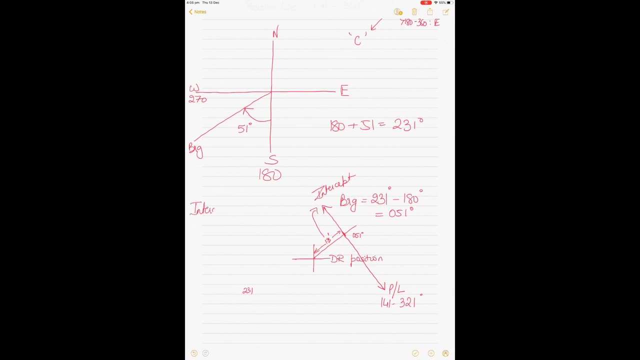 would be repeating myself a few times, but just watch what i did again. so what i did was that i used the three information that i had. i had the intercept right as 1.8 away, i had the bearing of 231 degrees true, and then, of course, i had the position line that 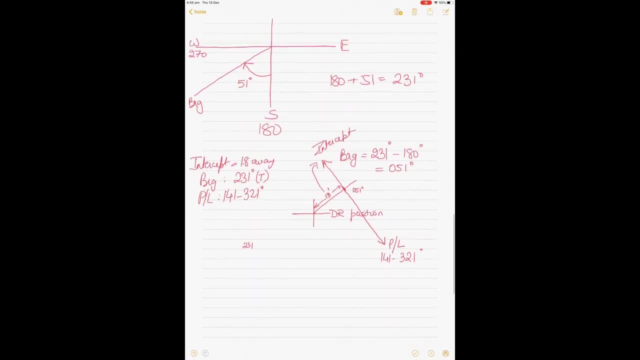 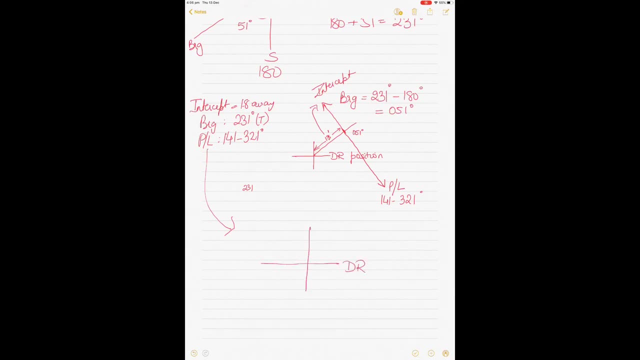 said it was 1412321. right, this is what i used. now what i did again and i'll show you here. right, this was my dr position, approximately dr positions, and because my intercept is 1.8 minutes away, that's 1.8 miles away instead of going towards 231. it would have been here if it. 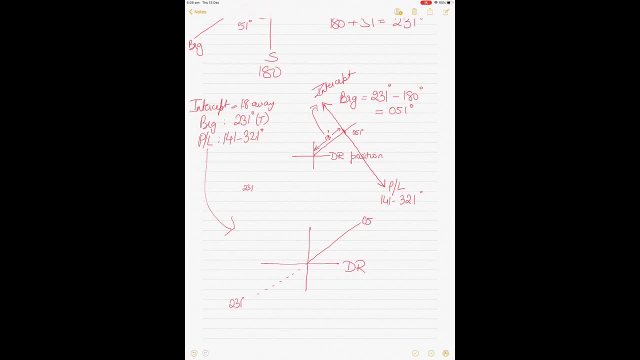 was a compass rose. i go towards 051 opposite to 231. this is 180 degrees away from it. i measure 1.8 miles on this line here and i mark it, and then i draw a perpendicular line. this is my position line. now, what does this mean? is this means that because i knew only? 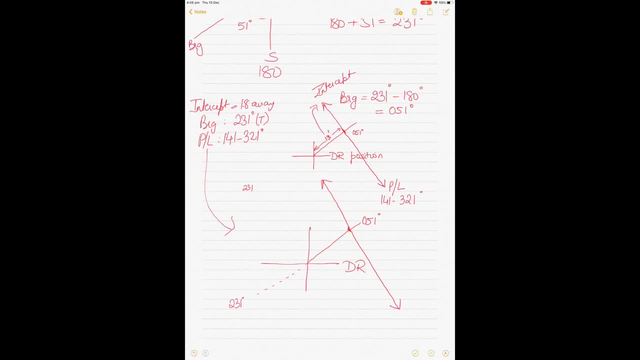 the dead reckoning position and approximate position at z when i took my sextant altitude from the sun and i've got my position line. what it does is basically gives me the bearing from the sun of the bearing from the sun could be. it could be, it could be a very long line. 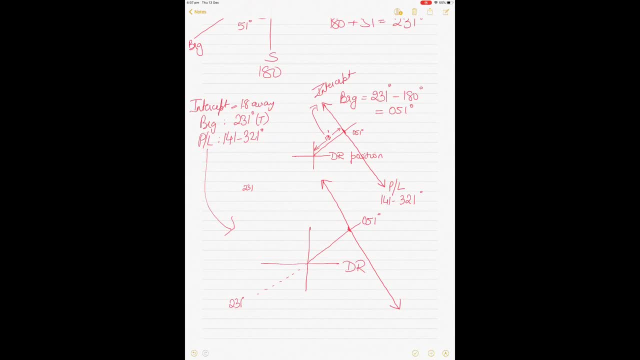 but because of these calculations, what we know is that our ship lies somewhere on this position line of 1412321. it lies somewhere here and through our calculations i know statistically i am somewhere very close to the intercept terminal point- this is called the itp, where. 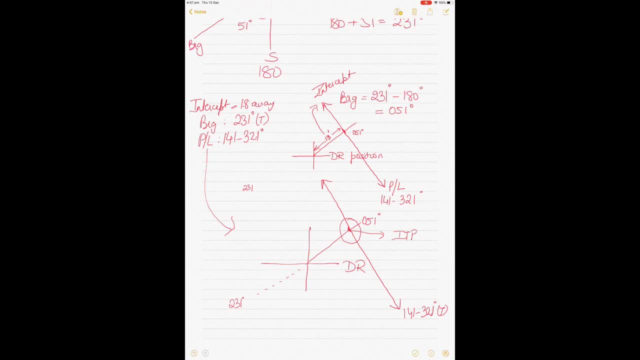 my intercept is cutting the position line intercept terminal point. all right, so what i need is: this is my position line. what i need is another position line from here, so the intersection of two position lines can then give me my ship's position at c. it's called a fix. now, in my next video, this is what i'll show you. i'll show you how. 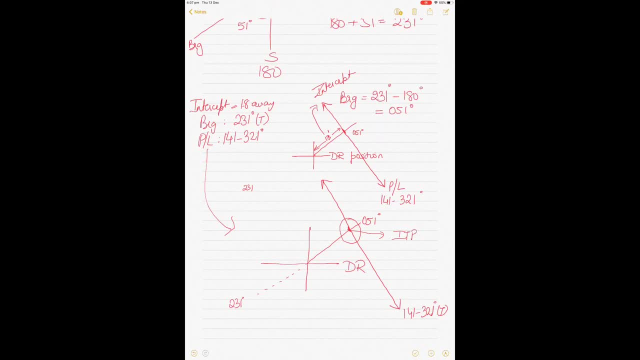 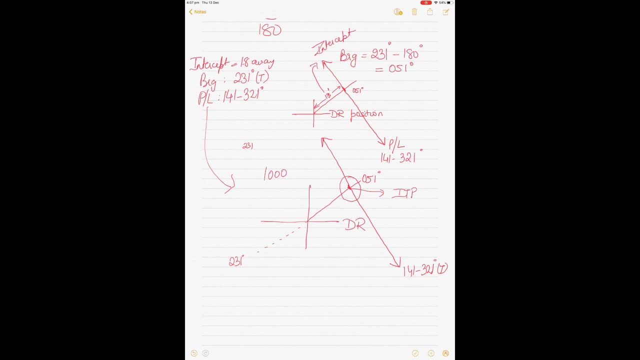 to plot the ship's position at c on the chart using two position lines. so normally what used to happen at c is that you take a position in the morning, say at about 10 o'clock, right, you get a position line intercept like that, and then you probably transit a few miles. 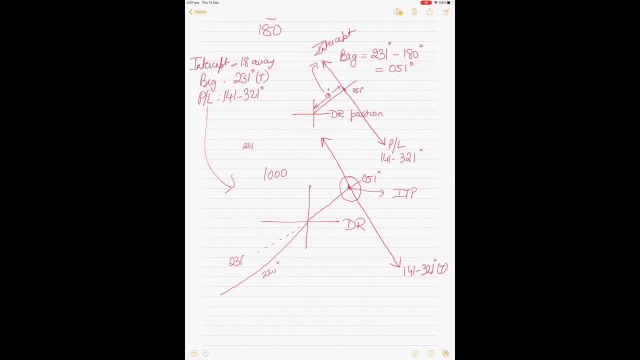 along a course- in this case, let's say it was on a course of two to zero degrees two- and you transit for till the noon position. you come at a noon position. you don't know where you are. you have caught your. you transfer this one here. right? you transfer this one. 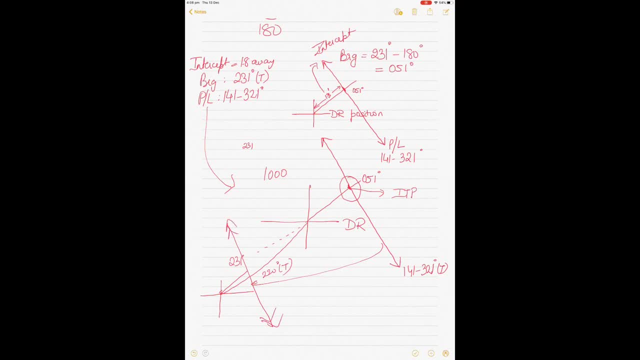 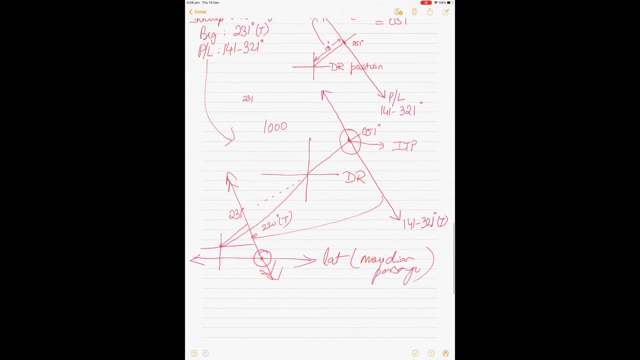 here. when you transfer it, you denote it by double arrows and then you get another position line. it could be a meridian passage, which gives you a latitude by meridian passage, or it could be another intercept end bearing the intersection of these two gives you your fix. so see, i won't worry too much. 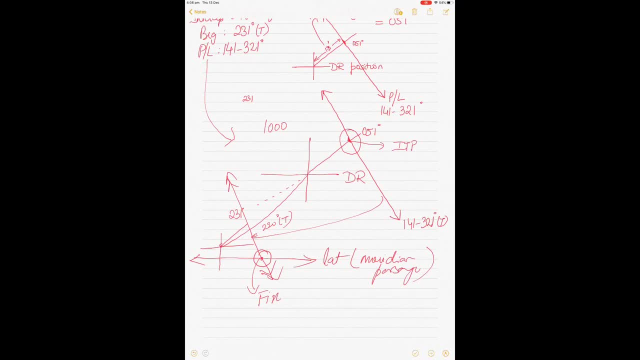 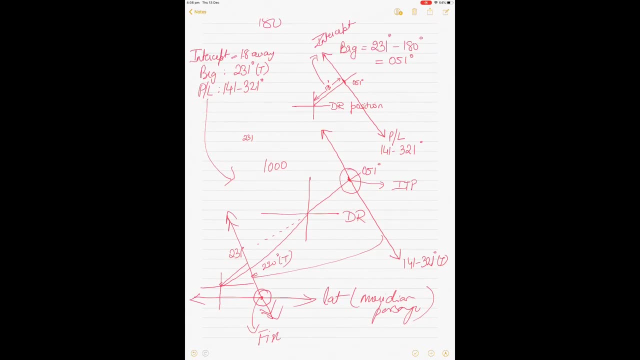 about this at this stage. this is just extra information i'm giving you all right. i was trying not to make this video very lengthy, but it is becoming lengthy here. i'm just giving a brief background here, but i'll show you more about this and i'll show you how to practically 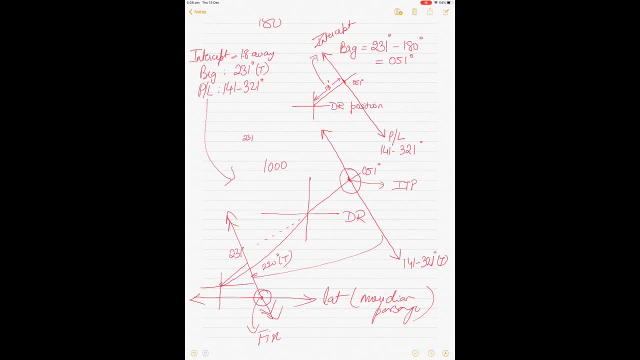 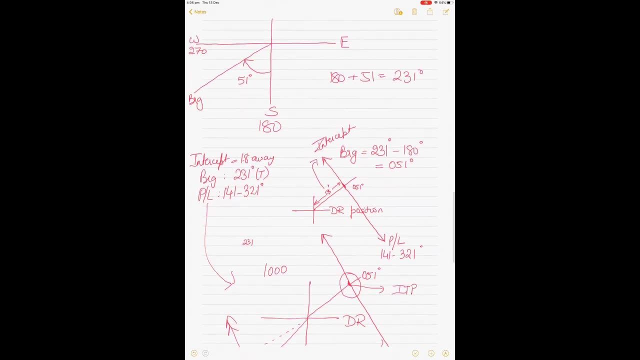 uh, plot it. how to practically use this information to plot the ship's position. uh, at c. all right, so don't worry too much about the later section, just go through it. if you want to go through it but focus more on the calculations above, see what i have done. go through it in stages. 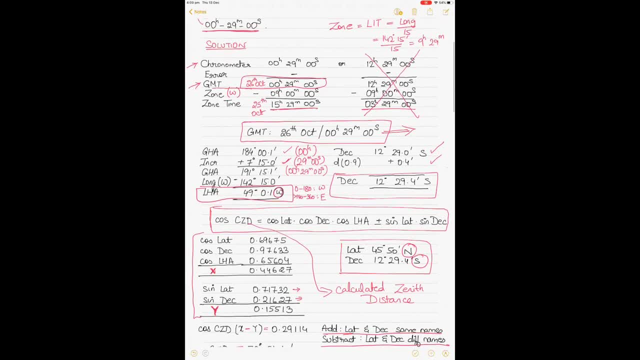 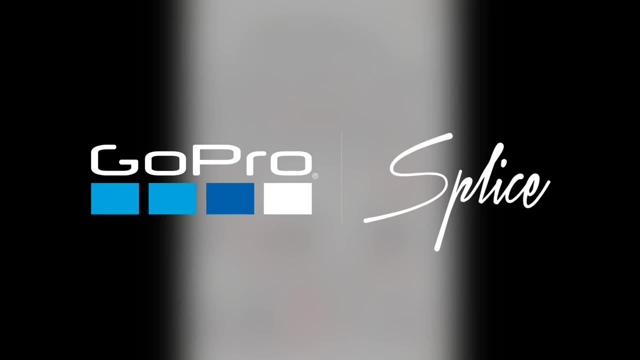 i have not wasted too much time on things that i've explained before in my previous videos, so make sure you watch it again and again to get a good understanding. all right, i'm happy to receive any questions through comments. thanks, guys.